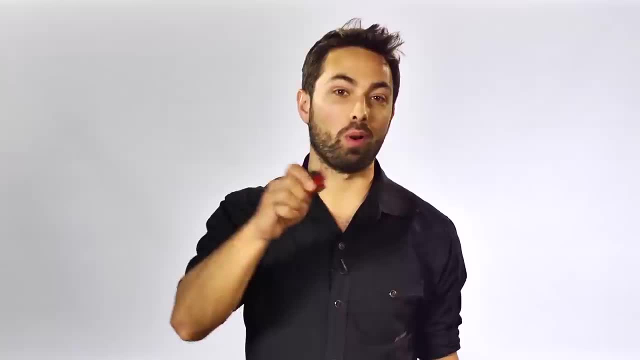 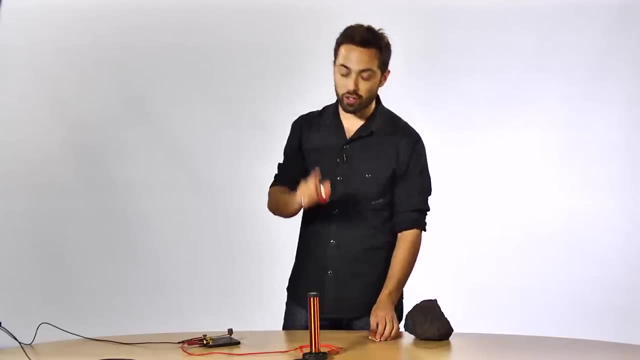 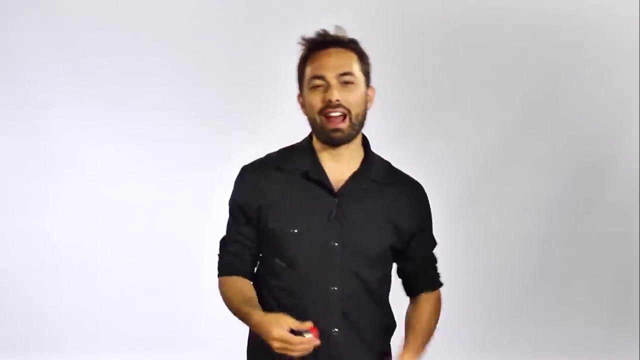 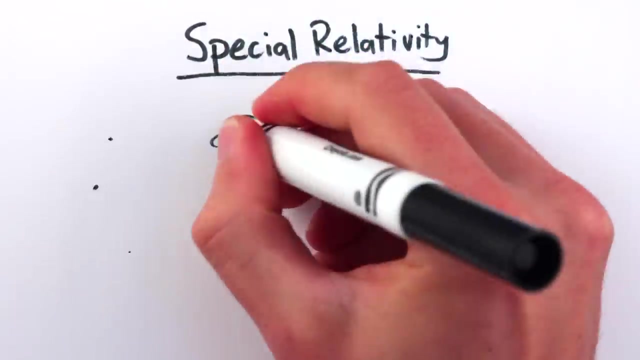 Only a few elements can be permanent magnets. Iron is one, Copper is not. But if you pass an electric current through any metal, it becomes a magnet, An electromagnet. But how does this work? Well, strangely enough, it's a consequence of special relativity. Special relativity is the 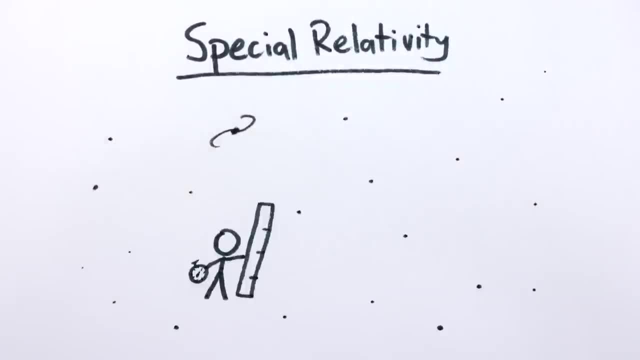 fact that in our universe, length and time aren't absolute. They're perceived differently by observers moving relative to each other, hence relativity. For example, if you measure carefully enough, you'll find that time passes slower for observers moving relative to you. Hey, Derek. 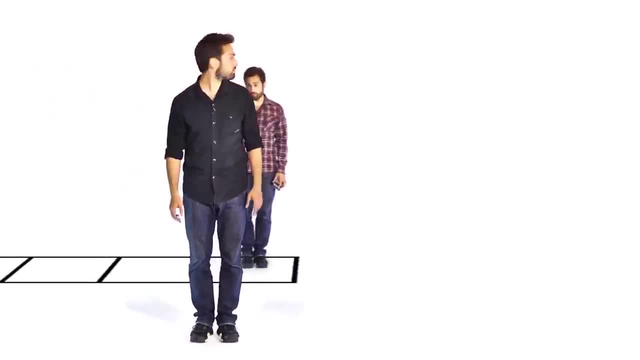 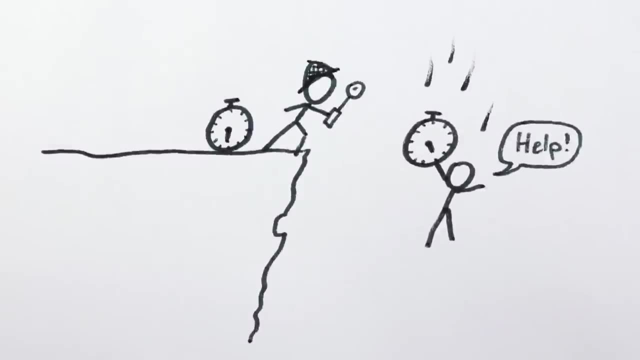 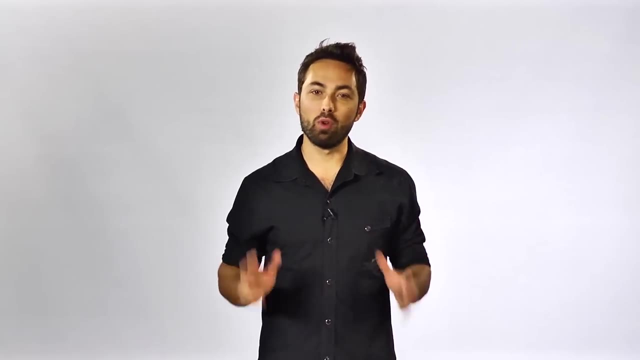 when did you last shave? Six hours ago, Actually, it was five hours 59 minutes and 59.999999999999 seconds. And moving objects are also contracted in their direction of motion. You're looking slim only in your frame of reference, So when an object is moving relative to you, it actually takes up. 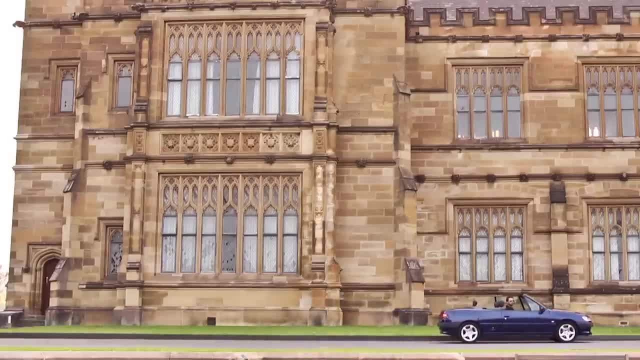 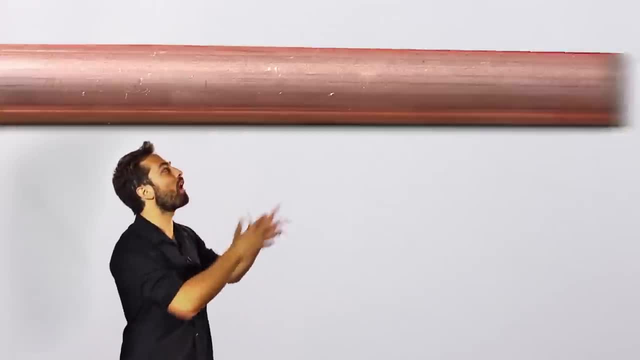 less time, Less space than when it's not moving, And even though this effect is obviously way tinier than we've shown. length contraction is what makes an electromagnet work. Picture a copper wire: It consists of positive metal ions swimming in a sea of free negative electrons. Now the number 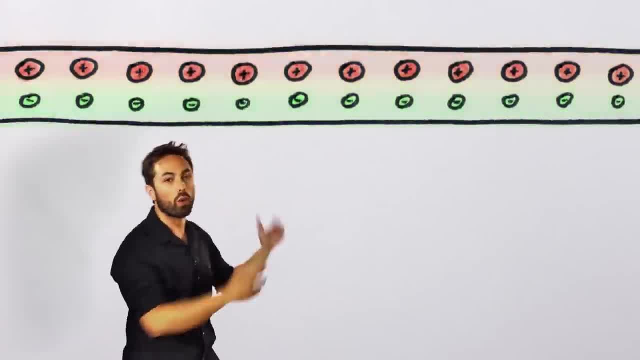 of protons is equal to the number of negative electrons. so overall the wire is neutral. So if there were a positive charge or positively charged cat nearby, it would experience no force from the wire at all. And even if there were a current in the wire, 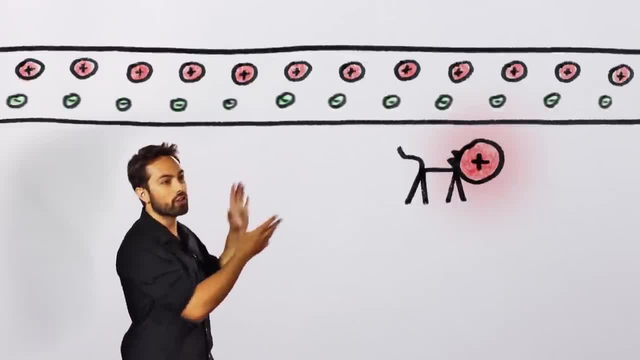 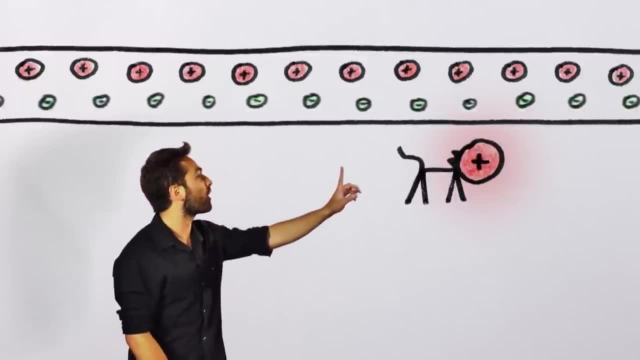 the electrons would just be drifting in one direction, but the density of positive and negative charges would still be the same, and so the wire would be neutral. so no force on the kitty. But what if the cat starts moving? Imagine, for simplicity, that the cat is moving in the same. 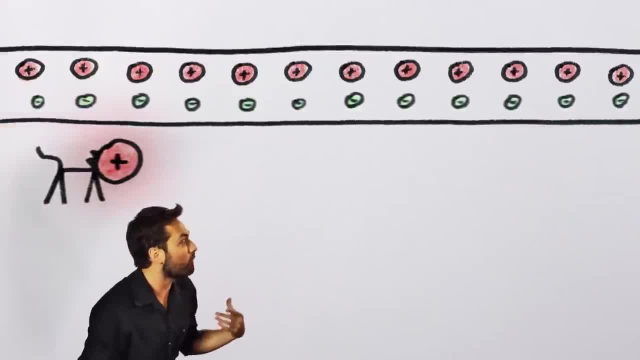 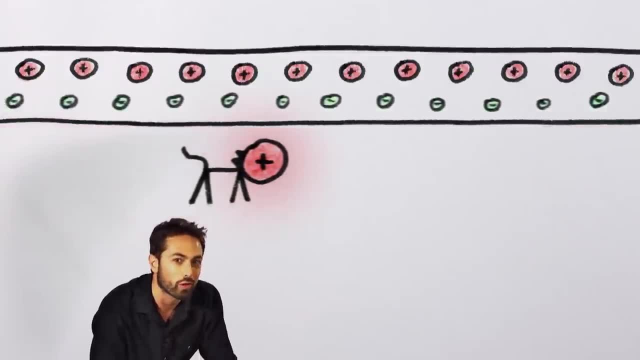 direction as the electrons, but the same velocity. Well now, in my frame of reference, the wire is still neutral and so there should be no force on the cat. But consider the same situation in her frame of reference. In the cat's frame of reference, the positive charges in the wire are: 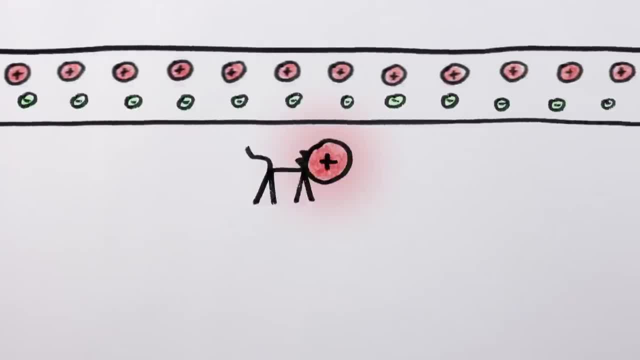 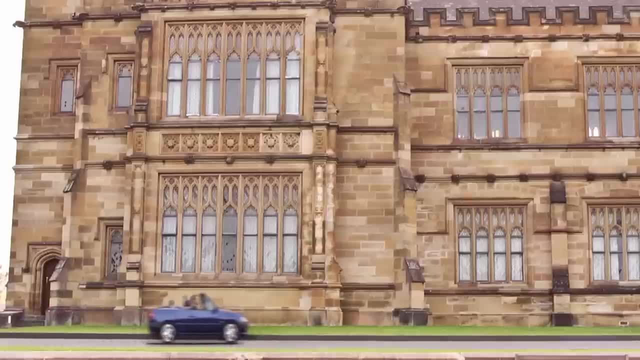 moving. so, according to special relativity, their separation will be ever so slightly contracted. Also, from this perspective, the electrons aren't moving, so they'll be more spread out than before. Remember, objects take up more space when they're not moving than when they are. These two changes